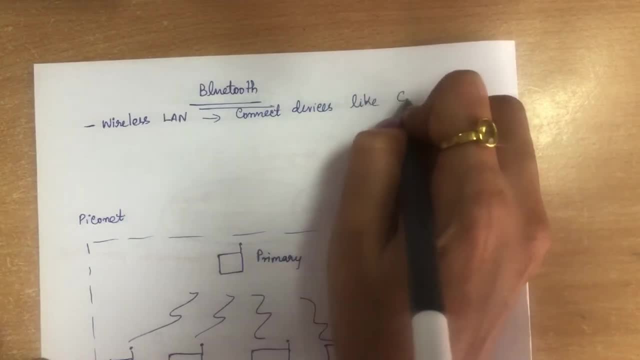 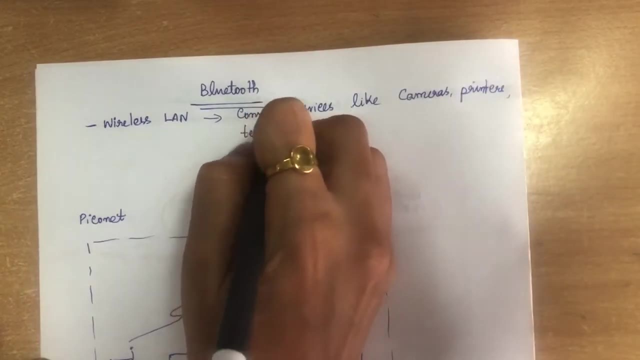 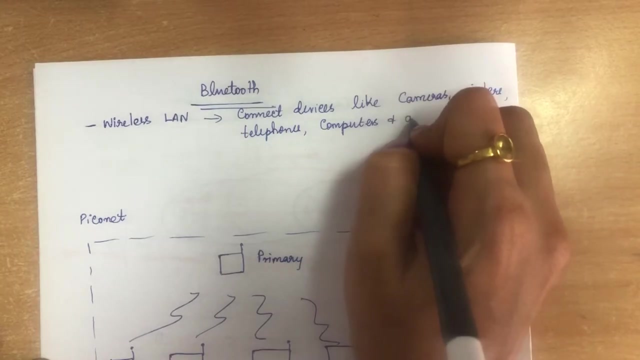 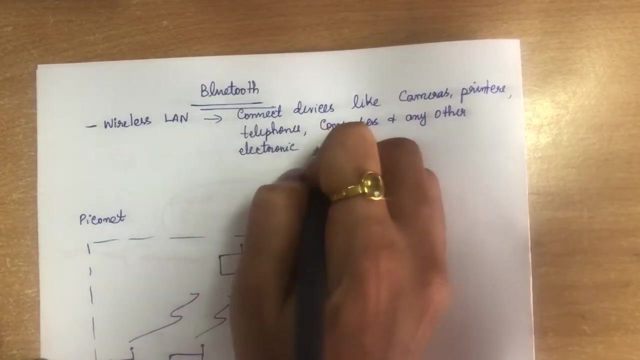 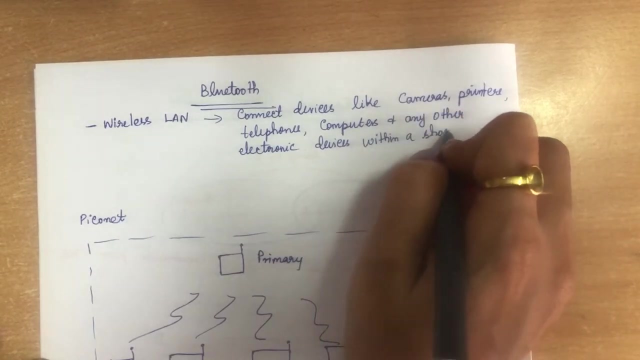 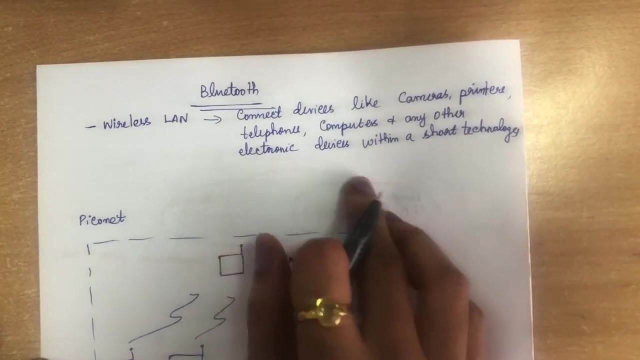 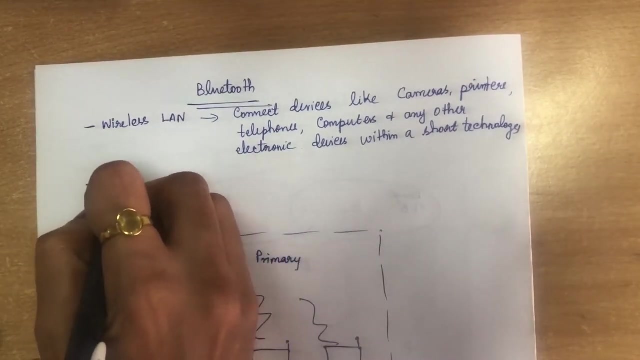 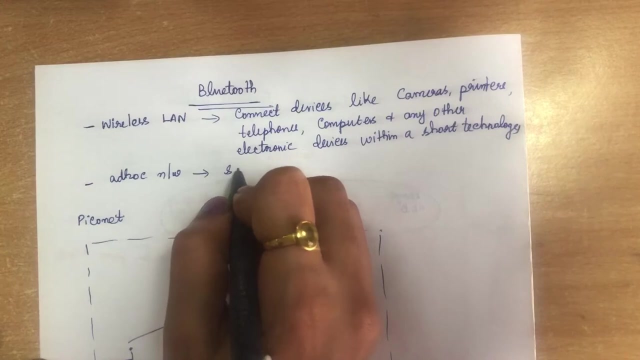 devices like cameras or even printers, telephones or computers or any other electronic devices can be connected. Electronic devices can be connected within a short distance. So using this Bluetooth technology, we can able to connect multiple number of devices. So if all these devices are within the range, we can able to connect the devices. This is called a Bluetooth. So we can say this: Bluetooth is nothing, but it is an ad hoc network. Ad hoc network, which means that the network is formed spontaneously, So we can able to create the network spontaneously. 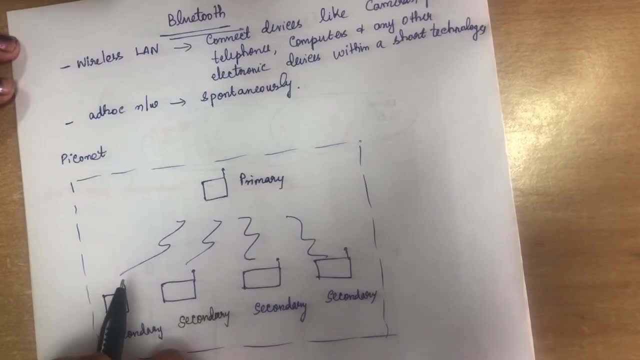 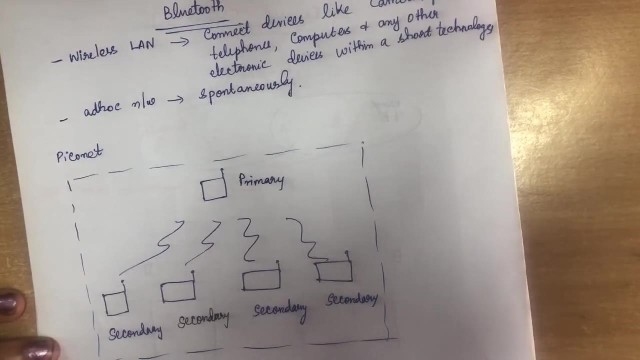 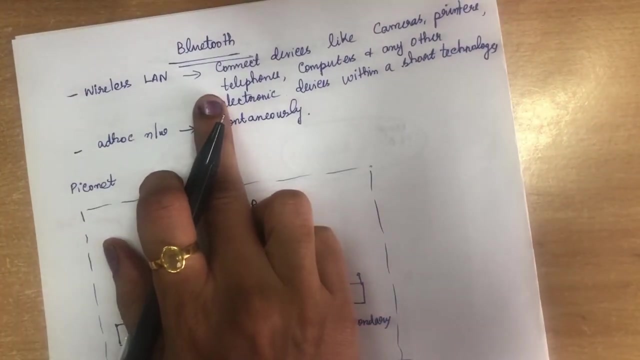 Even if you use Bluetooth technology, though, it can be connected with these gadgets also. Bluetooth technology, it has various applications. Nowadays, we people, we are using so many different applications in daily life. So, for example, we are using our wireless keyboard or wireless mouse Or careless mouse, and we are using our so many home gadgets Also. it has been connected with Bluetooth devices. So all these applications, they are using this Bluetooth technology only. So this Bluetooth technology was defined in the IEEE standard. 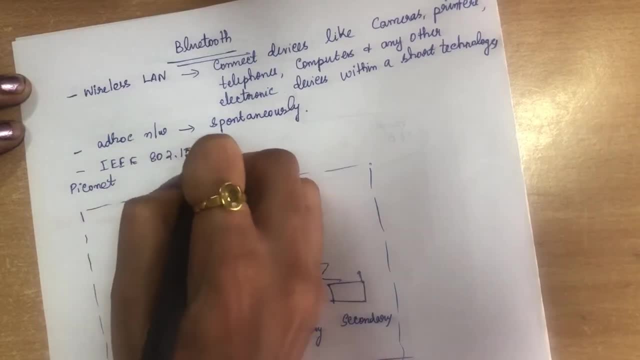 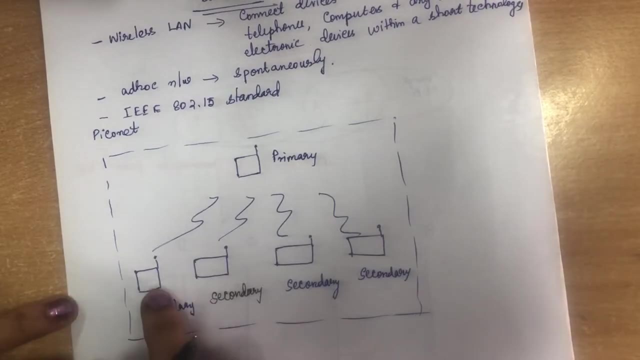 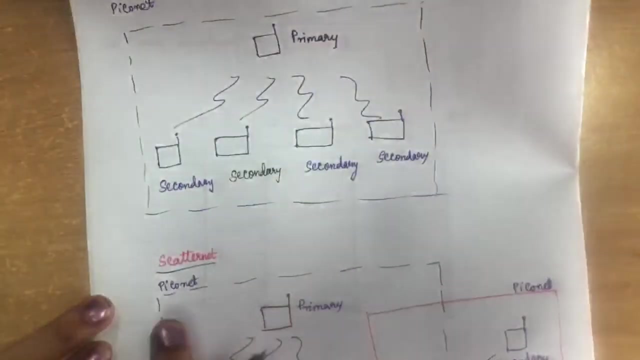 standard 802.15. so it was. it is defined in the standard call 802.15. so next we will see what type of networks you have in this bluetooth. so the first type of it offers two types of networks. one is pico net, other one is scatter net. first we will see what is pico net. in case of pico net, 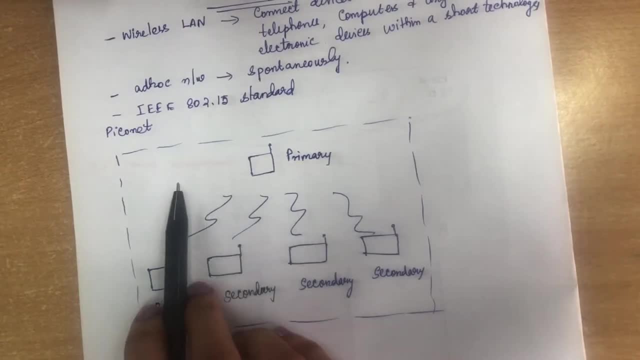 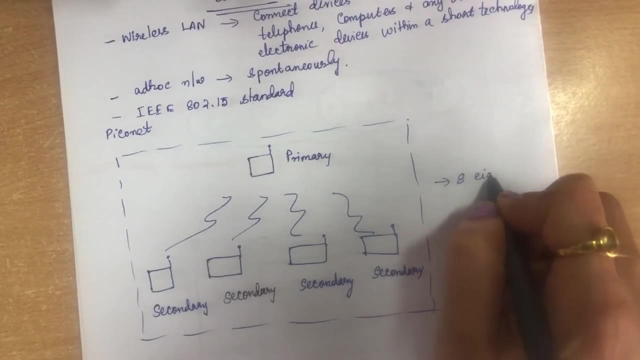 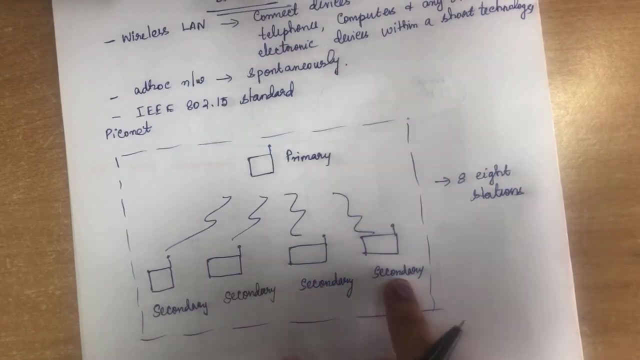 so there will be all the stations. it will be a bluetooth network. you can call it as a small net. so pico net can have up to eight stations. it can have up to eight station and one of the stations will be the primary station. so one of the station will be primary station. other stations will be 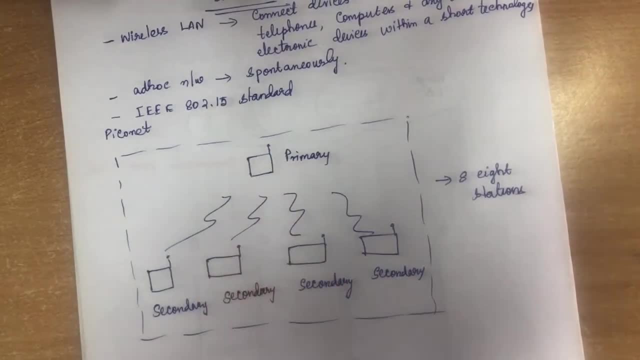 secondary station. only primary station can communicate with the secondary station, so we cannot able to connect. all your secondary stations cannot communicate. only primary station can connect. so total number of stations inside your pico net will be eight. so eight is the number of number of stations inside your pico net. so pico net is the number of stations inside your pico net. 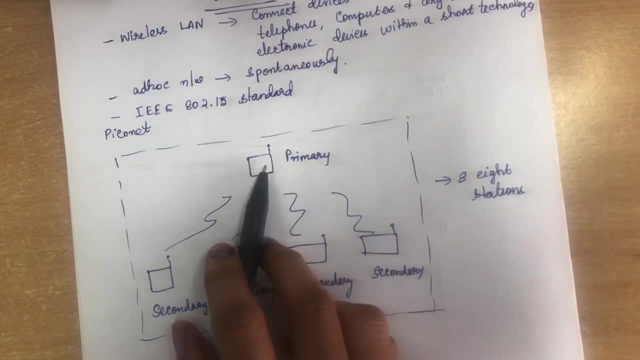 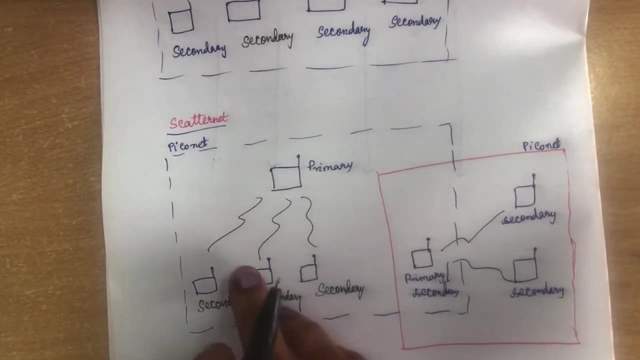 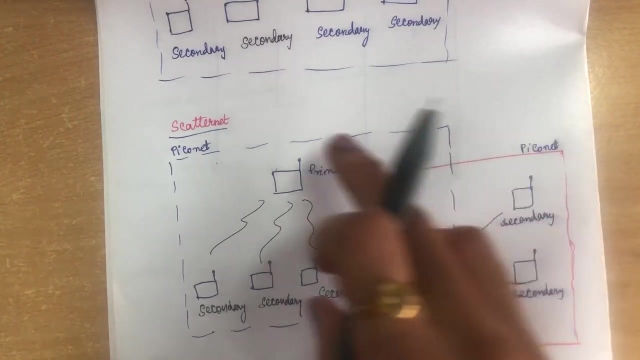 is eight. so only primary station can able to send data to secondary stations. okay, this scatter net. so in this scatter net. so number of the pico nets can be combined to form the scatter net. so what happens? you can see two pico nets. it is combined to form the scatter net over here. so here you can. 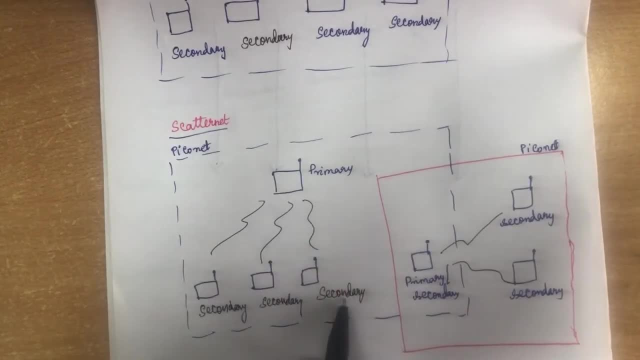 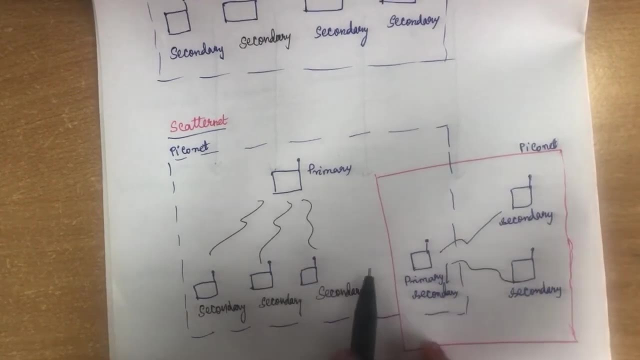 see one pico net where you have a primary station, other stations or secondaries, and you have one pico net over here where you have primary station, and these are all secondary stations. so what happens is that is this, this primary, this secondary station, in this primary it act as a. 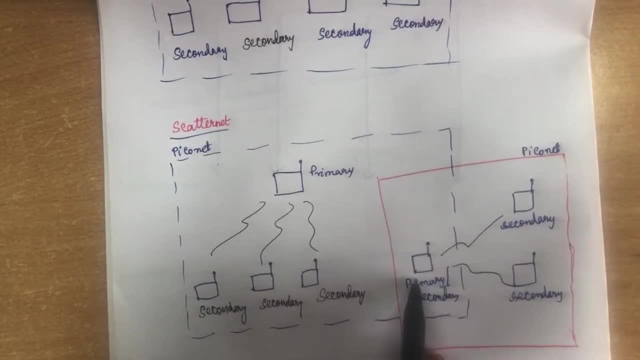 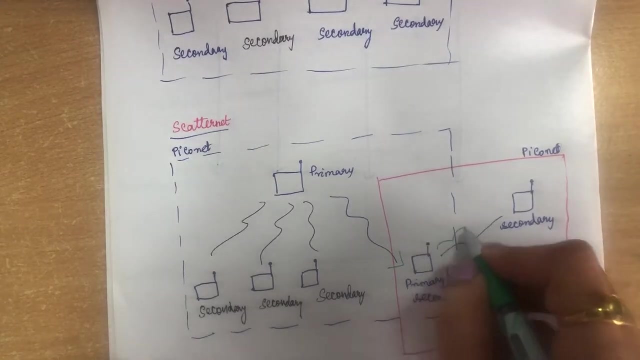 primary station in second pico net. so what this station will do is, first, it will get the message from this primary station, the secondary station will get the message. it will get the message from this and, after getting the message from primary station, this will act as a primary and it will. 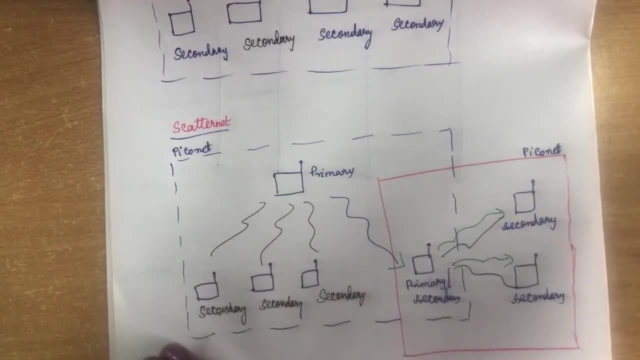 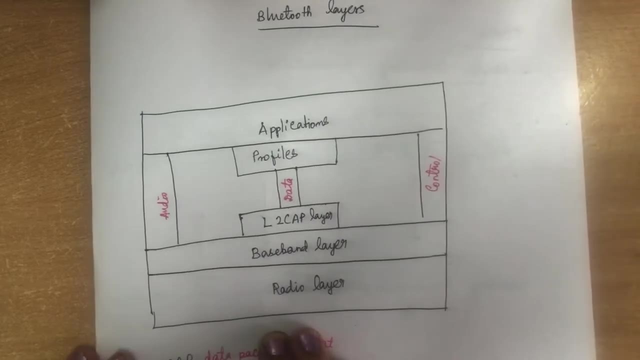 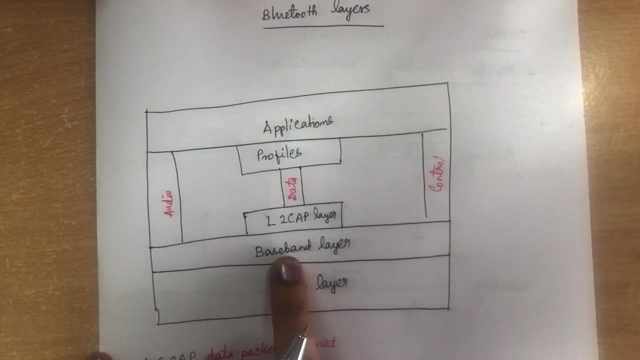 send the message to another pico net, so this process is called a scatter net. okay, coming to the bluetooth layers. so this bluetooth layers is somewhat different from your, from your tcp protocol, osa protocol, so what we have is radio layer and then we have baseband layer. 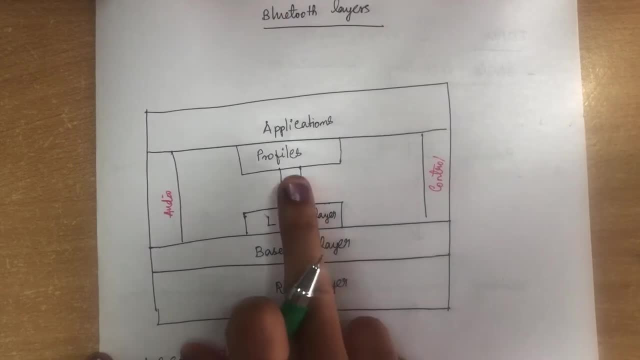 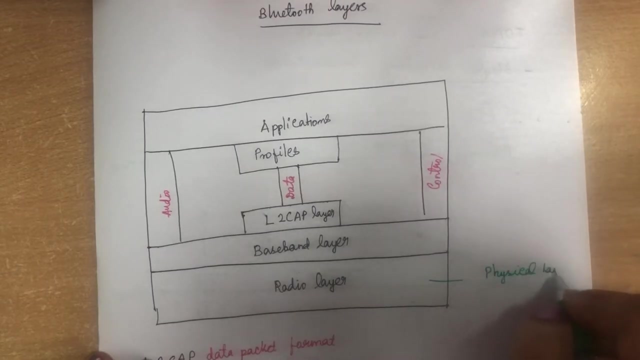 and the next layer is logical link control adaptation layer and we have profiles this side, audio and data control and applications. so this is an architecture of your architecture of bluetooth layers. so this radio layer is somewhat similar to a physical radio layer layer in osa model and this base band layer is similar to a max sub layer. it is it represents. 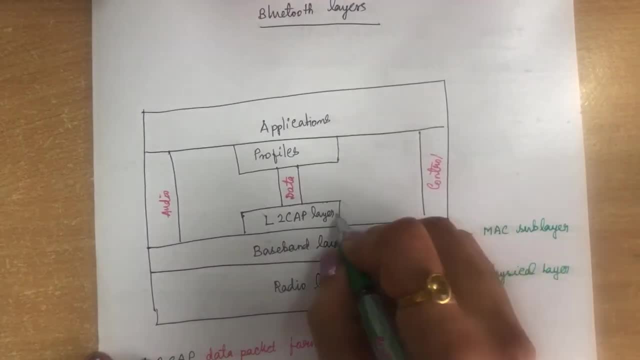 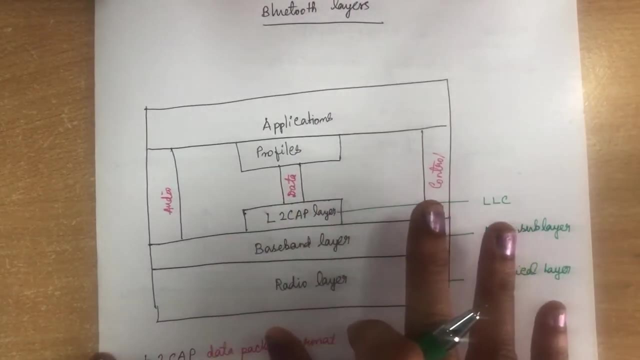 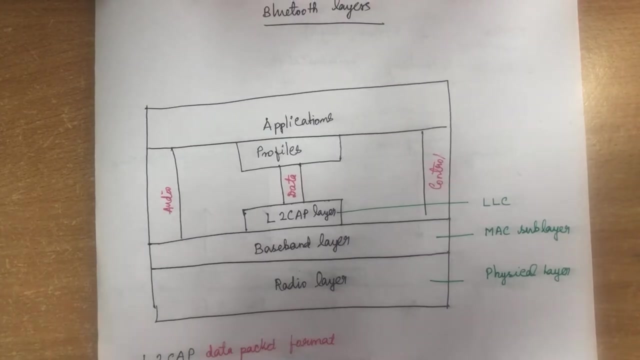 a max sub layer. okay, and this logical link control layer is also a logical link control sub layer in data link and you have application. so these are, these are all the protocol layers. so which is which is totally different from the iso osa layer or tcp protocol suit. next we will. 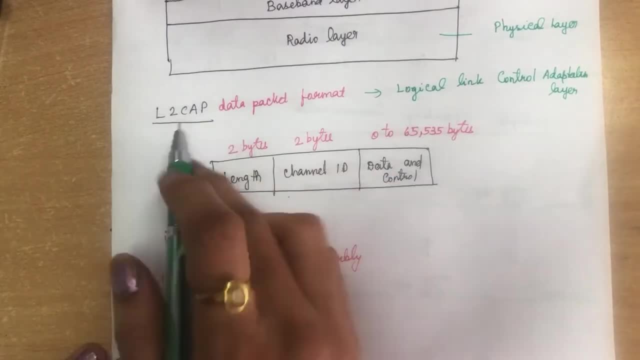 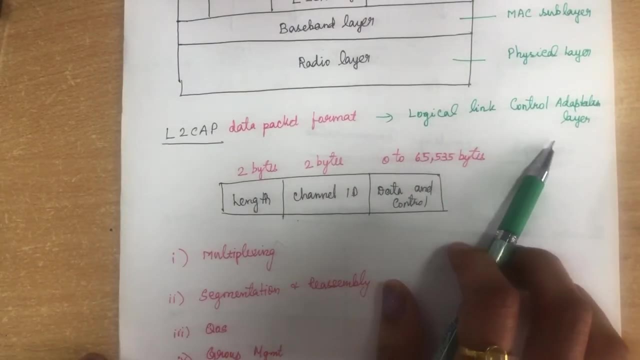 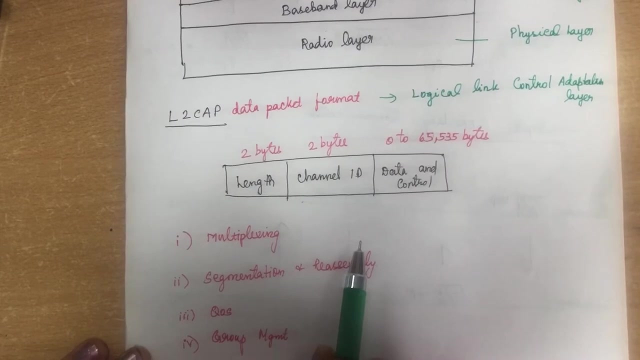 see in detail. on logical link control adaptation layer: l2 cap is nothing but logical. this l2 cap, that is nothing but logical link control. adaptation layer, this layer layer, sub layer, is similar to what we have in logical link control in tcp, ip or it can be in logical link control. that is like: 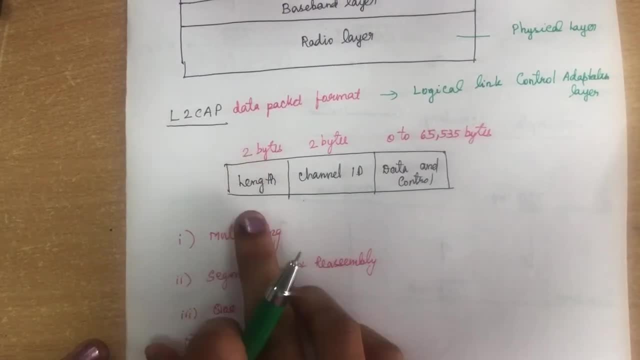 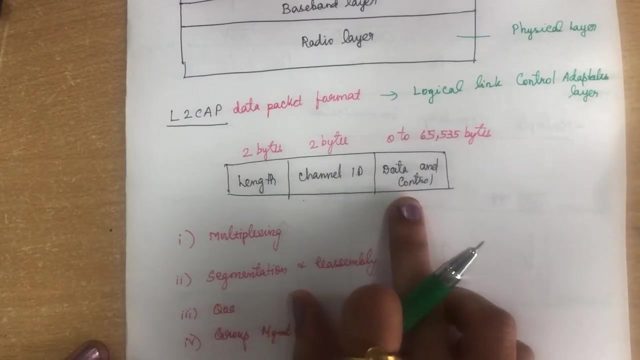 or in iso ac layer. so, coming to the frame format of logical link control, first we have the length, that is, this length will define the size of the data which we receive from upper layer, and channel id is used for creating the virtual channel. it is a unique identifier for that particular data. and then we have the data, so the data will be. 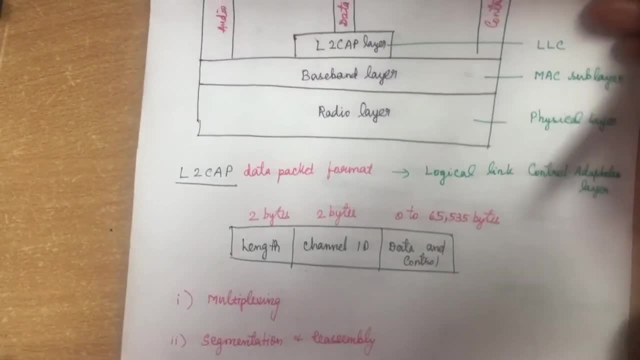 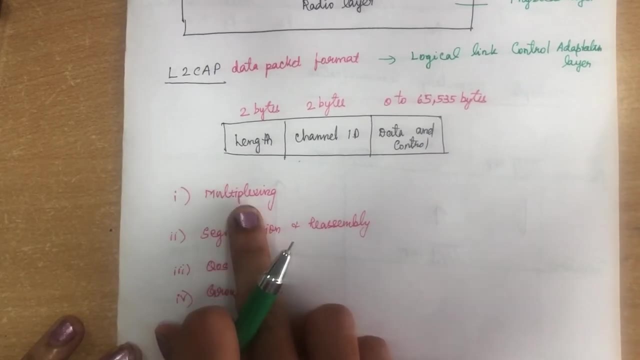 within the size 0 to 65 535 bytes. so this is the, the frame format of logical link control adaptation layer. so what are the functions which is performed by logical link control is multiplexing. multiplexing what it does? it has to accept the data from the upper layer. it has to 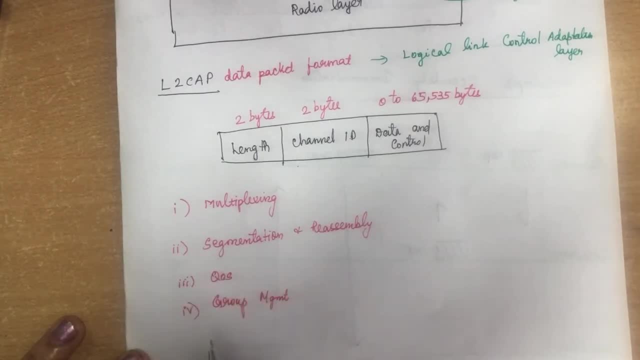 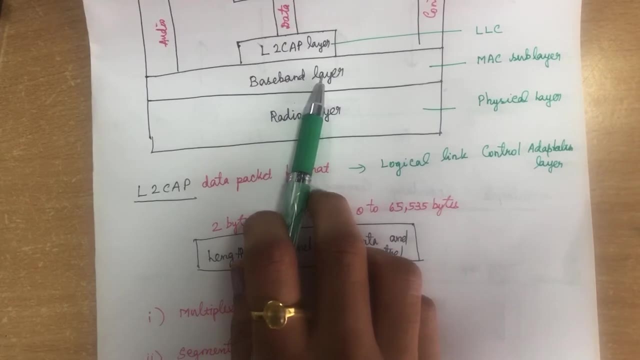 that is like it puts. it frames them, then it gives us to the baseband layer, so how assembly and reassembling is encapsulating or decapsulating is done in data link layer, so logical link control. it puts everything into a frame and then it will. 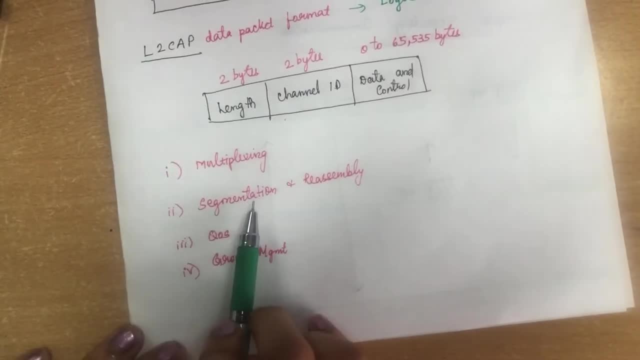 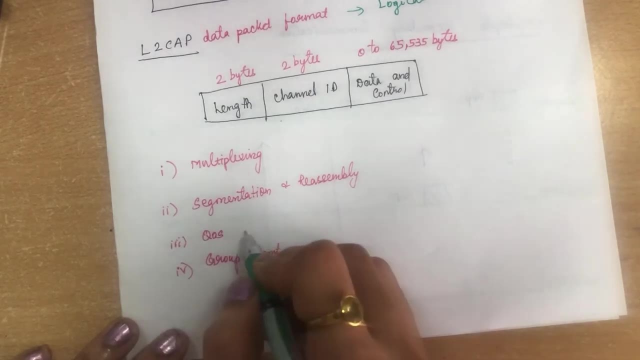 send the data to lower layer. that is called multiplexing. segmentation, reassembly is also one of the work of this logical link control and also it does. it has to maintain best quality of service is maintained through the transmission, best qos is given and it also ensured that there will be a 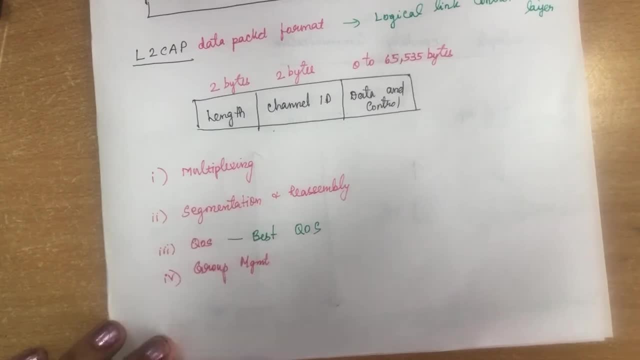 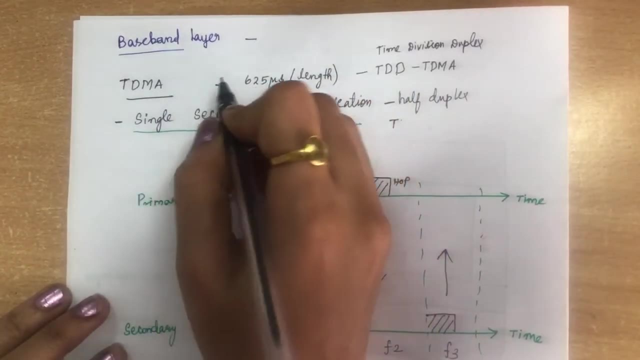 protection between all the devices inside the pico net. ok, these are the functions of logical link control adaptation layer. we will see the baseband layer, so coming to the baseband layer of this Bluetooth protocol. so coming to this brood, to technology, this baseband layer. it is similar to a. 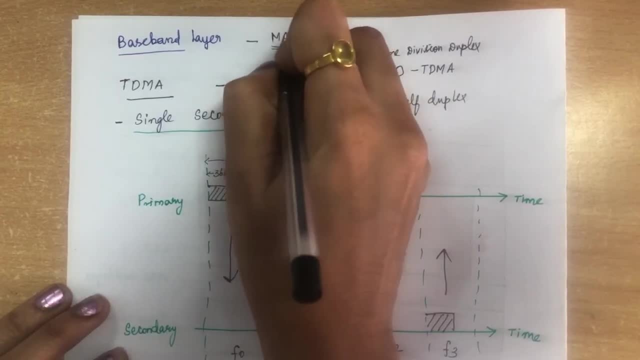 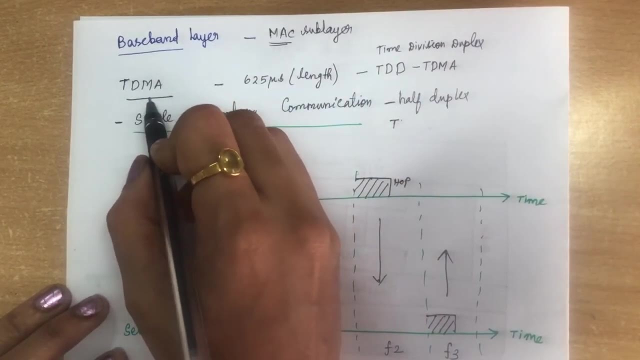 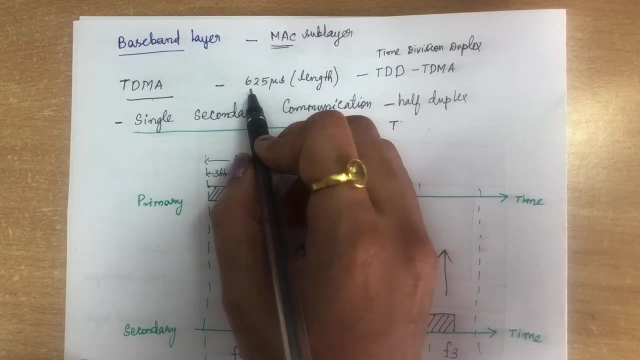 math sub layer. ok, in math sub layer what we have? all this thing. it is same, similar to this. the access method used is TDMA- time division, multiple access. so here what happens is we are going to divide into time and we are going to use the channel. so length of the time slot is: 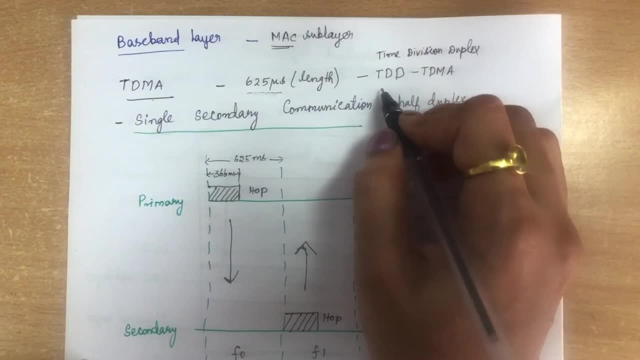 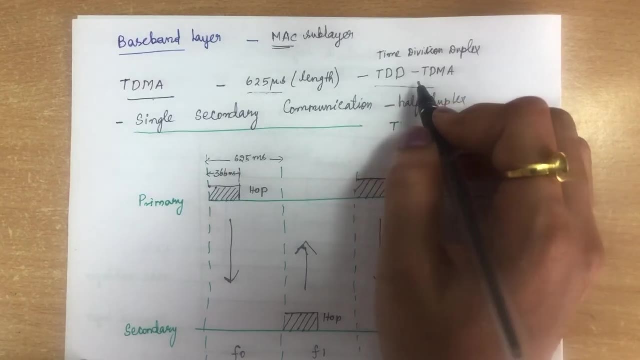 actually 625 microsecond, so it uses a format called tdd, tdma, that is time division duplex, tdma. so what do you mean by time division? duplex is when sender and receiver wants to sender. both sender and receiver can able to transmit, but not at the same time. this is called time division. 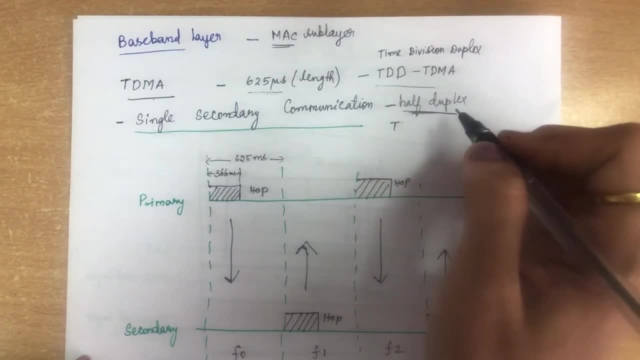 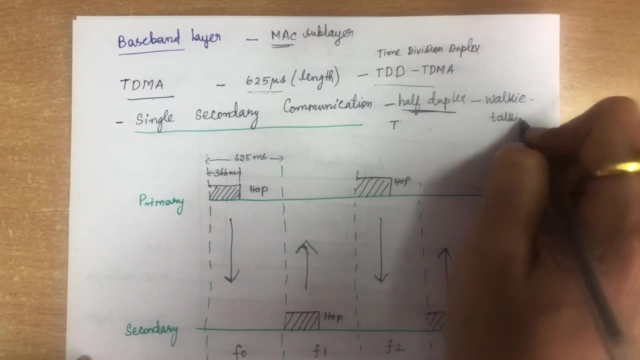 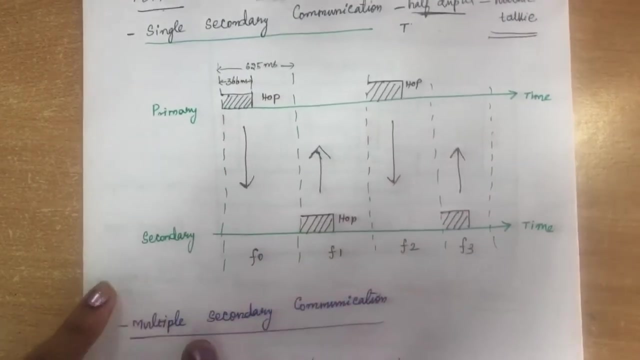 duplex. this is similar to an off duplex. so this technology is similar to a walkie talkie. so how we use a walkie talkie, so in walkie talkie at the same time. both cannot able to speak or communicate. so it works in two communication mode. one is single secondary communication. other one is 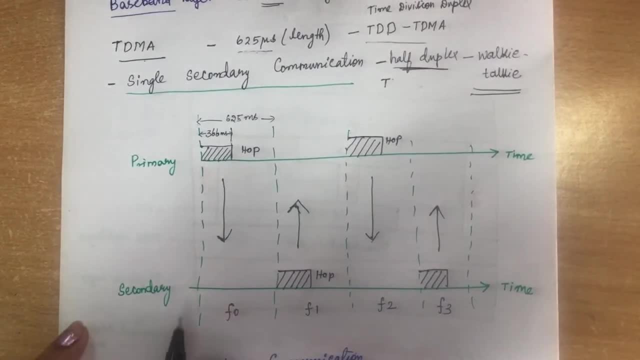 multiple secondary communication. coming to single secondary communication, you think that there is. it is the tdma. concept is very simple in case of single secondary. so you have one of the two types of communication, which is the one of the two types of communication, which is the one of the two types of communication, which is the one of the two types of communication. 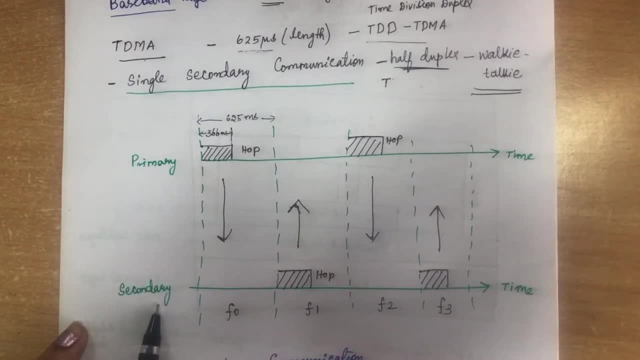 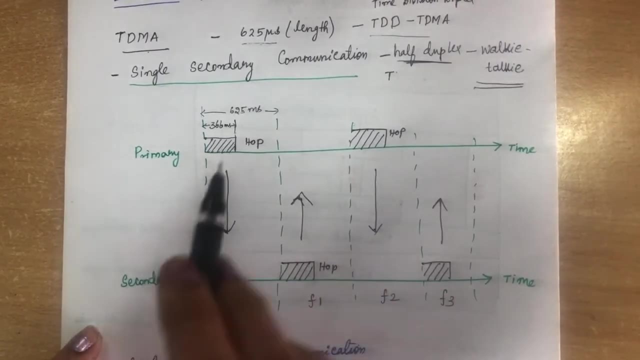 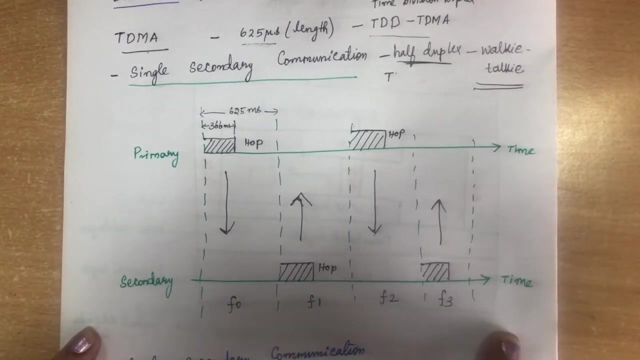 only one primary station and you have only one secondary station, so it is tdma. concept is very simple. so here the time is divided into so many: 625 time slot is total, time slot is 625 microsecond and and it has been divided into so many time slots so primary station can use even number slots. 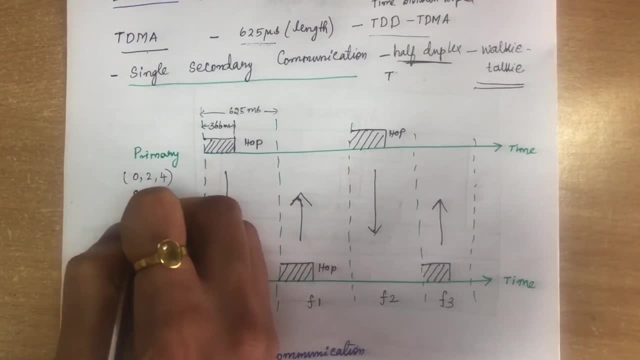 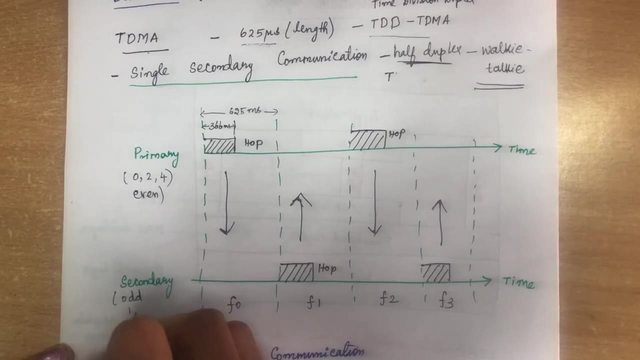 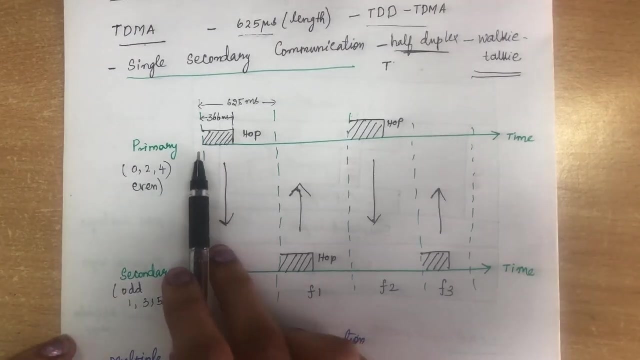 like 0, 2, 4, even- it uses even number slots and all your, all your secondary station will use odd number slots and all your, all your secondary station will use odd number slots. so like 135. so it uses all secondary station uses odd number slots. so in this you can see this when primary station wants to. 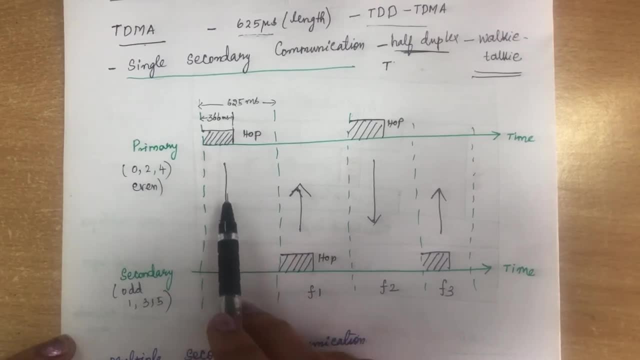 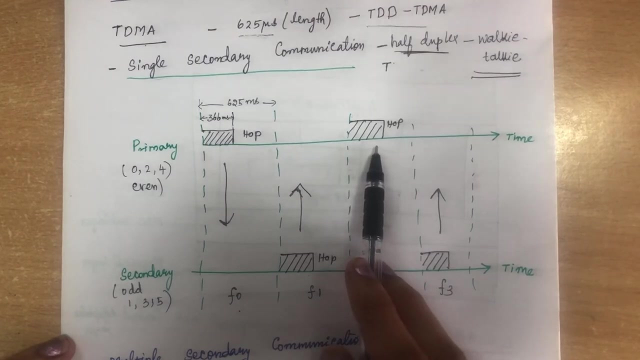 send the data it uses. it sends a data in even number slot F, naught and the next. when secondary station wants to send, wants to send the data to primary station, again it can send it in the odd numbered slot called F1 and again primary station can send it in the next time slot and then it can. 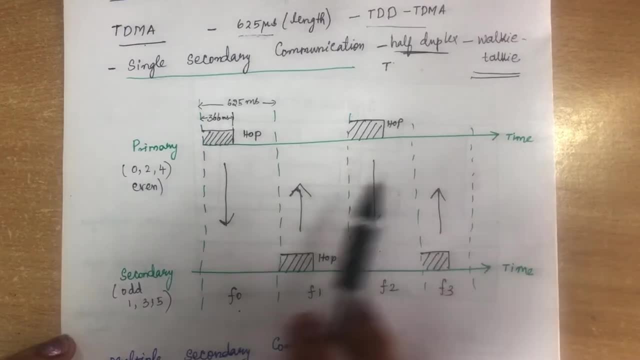 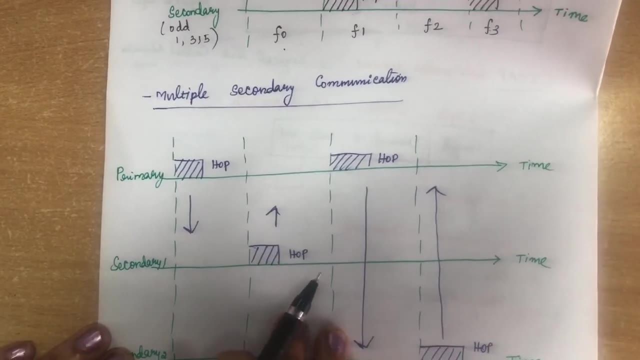 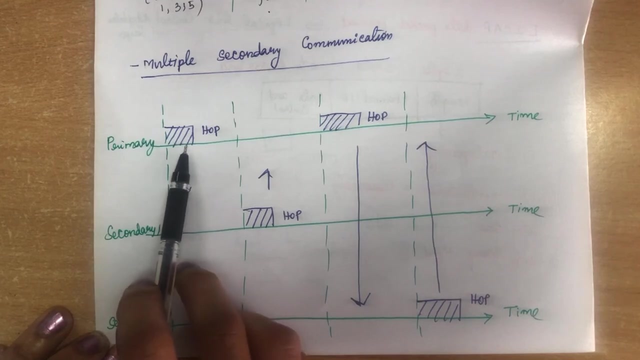 secondary station will be sending it in the F3 slot. This is how the communication takes place. in case of single secondary communication, Multiple secondary communication, you can see there is one primary and you have multiple secondary devices. So in first time slot the same thing it has been. the time is divided into 625 microsecond and primary station will use all. 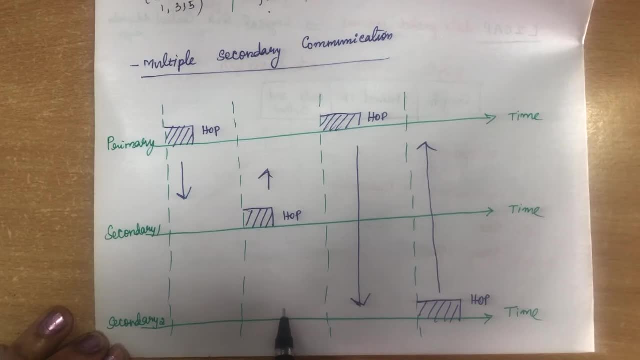 your even numbered slot and secondary station will be using next odd numbered slot. So primary station: first it will be communicating with secondary 1 and now secondary 1 will be communicating with primary 1.. Now primary 1 will be communicating with secondary 2 and secondary 2 will be sending. 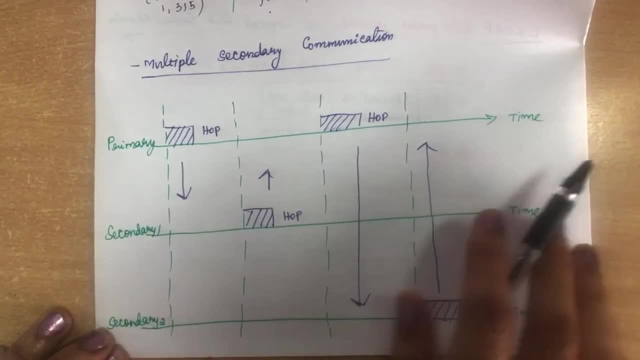 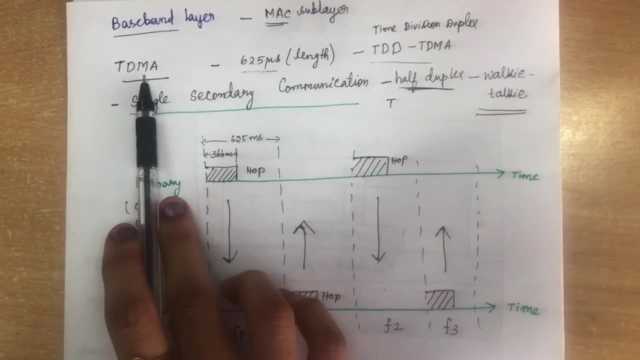 the message to primary 1.. So this is primary station. This is how communication takes place in multiple secondary communication. So the baseband layer it uses TDMA concept. Its access method is time division, multiple access, but in that it uses time division duplex, that is like 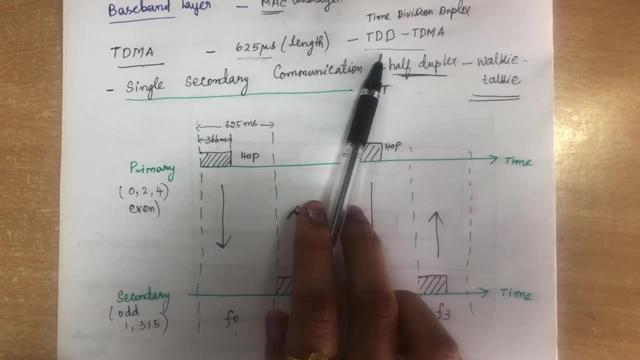 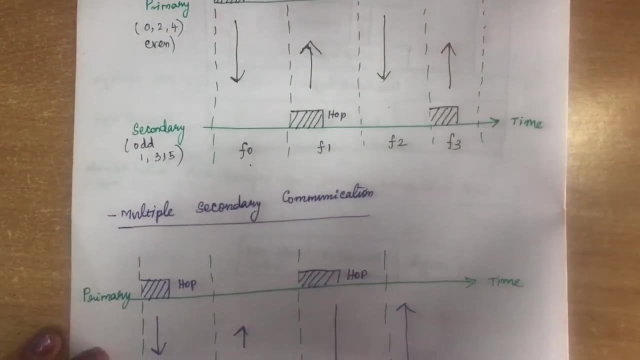 it can. both the sender and receiver can able to transmit, but not at the same time. So it uses single secondary communication and as well as multiple secondary communication for transmission. ok, So next comes the frame format of baseband layer. So frame contains the format structure. 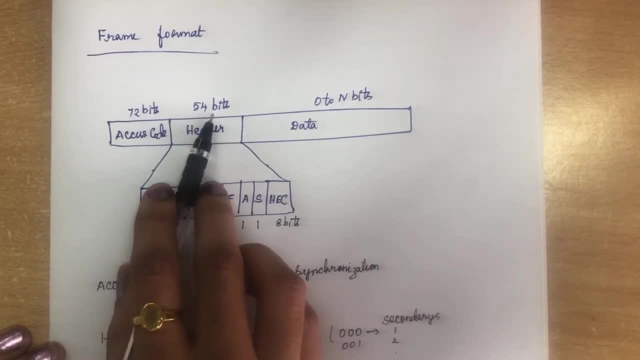 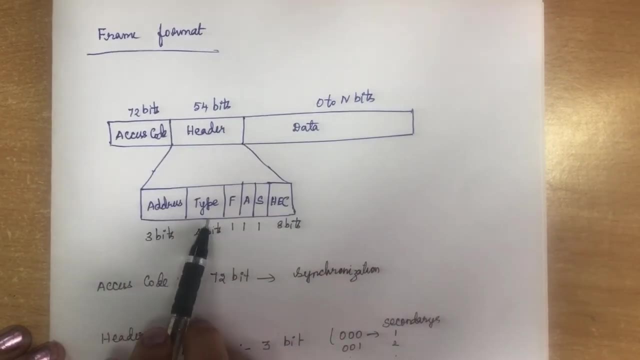 is access code which is of 72 bits, and then it has a header which is of 54 bits and last it has a data of 0 to n bits. Coming to the header, it will have sub fields like address type, F, A, S and H E C. 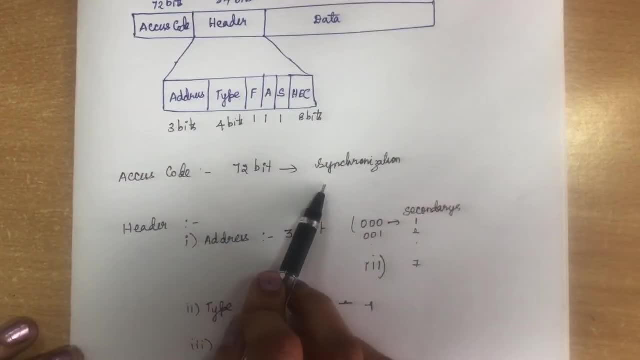 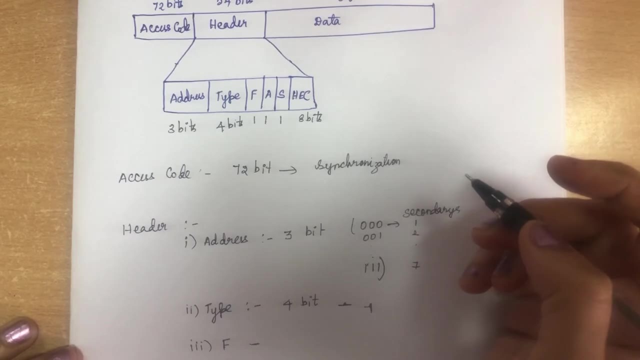 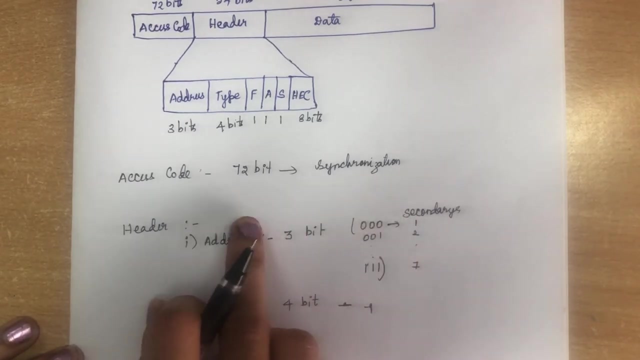 Coming to the access code, It has 72 bits. It is used for synchronization. This is similar to that is preamble in preamble, how we have used in standard Ethernet. So this will: this is used for synchronization purpose. This will alert the receiver that it is going to send the data afterwards. Ok, 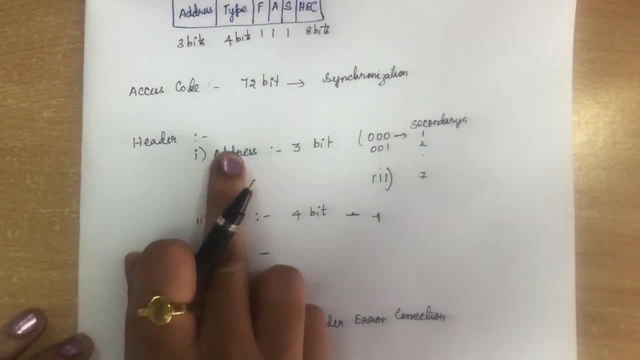 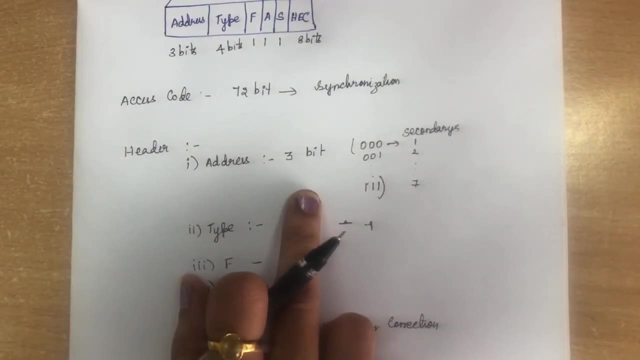 Next is header field. Header field- it is of 54 bit, So the first three. first is an address sub field we have in this header So which is of 3 bits. So this will define the secondary devices. So 3, it is of 3 bits, which will define usually in the piconet we can have. 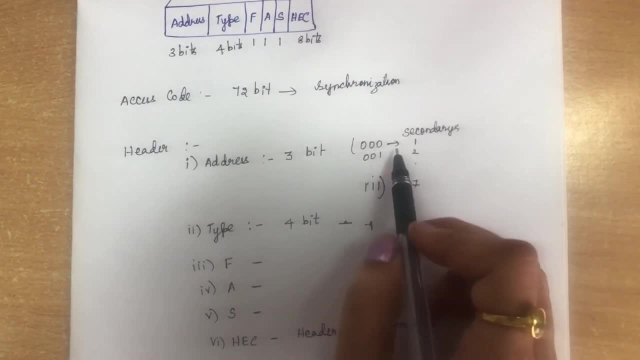 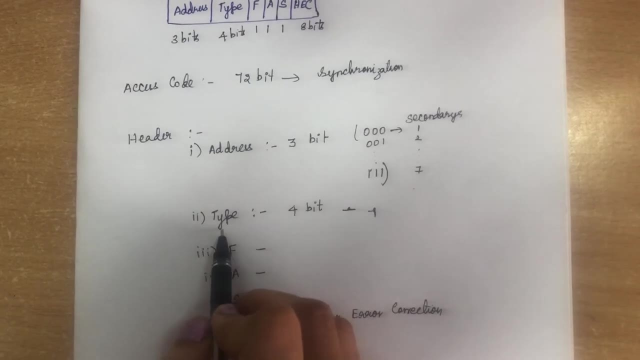 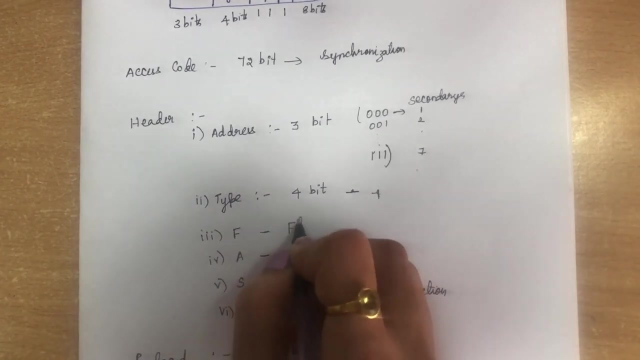 only 7 secondaries. totally 8 devices are there. So which will represent this 3 bit will represent the secondary 1, 2, 3, up to 7.. Ok, Next is type field represent the type of data we are going to receive from the upper layer, and F field is nothing but flow control. So when this 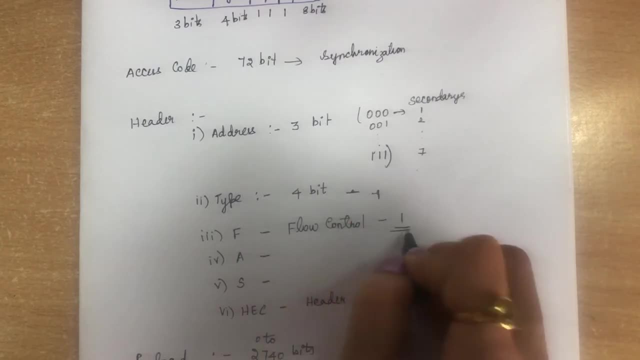 field is set to 1. this is a 1 bit field. When this bit field is set to 1, that means that buffer is full. So this is a 1 bit field. When this bit field is set to 1, that means that buffer is full. 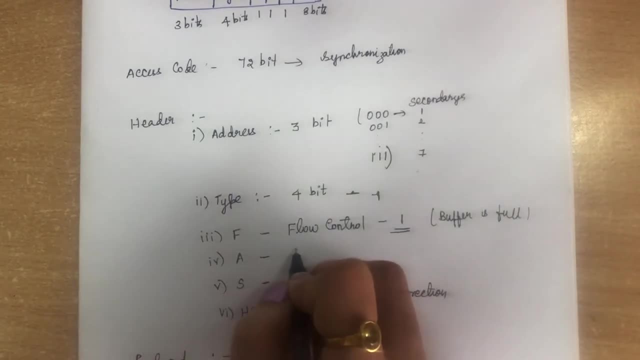 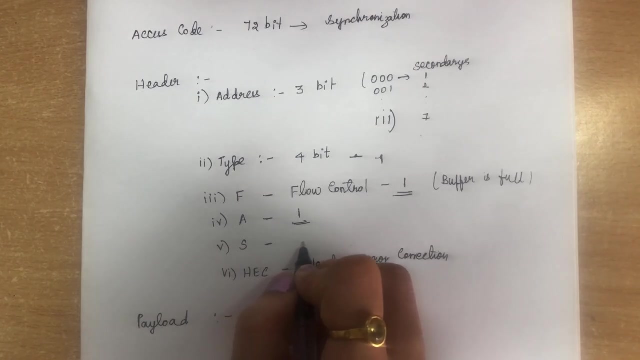 Ok, and next is A is for acknowledgement. When this bit is set to 1, it represent the acknowledgement field. and next is S field, it represents your sequence number. and last is HEC. that represent header error correction, So which is of 8 bits, So which is used to.